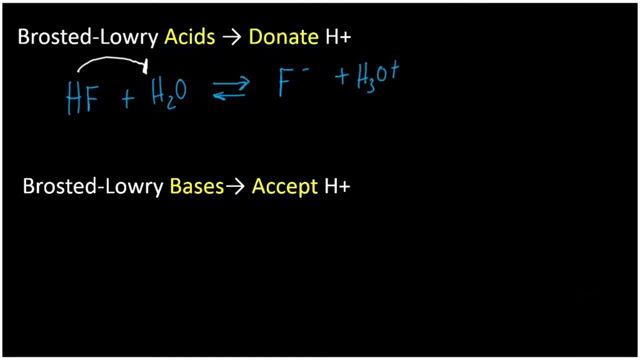 when it gained a hydrogen ion. So there we have our Bronsted-Lowry acid. So I'm going to label that our BL acid. All right, now let's look at a Bronsted-Lowry base. One example of a Bronsted-Lowry base: 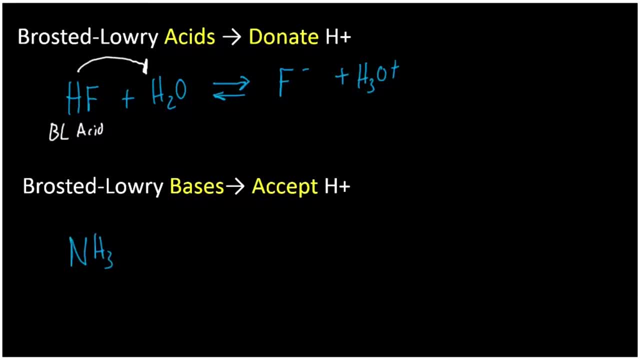 probably the most common one is NH3,, which is ammonia. When we react it with water, we know that because it's a Bronsted-Lowry base, it's going to accept a hydrogen. That means that the hydrogen is going to come from water and be transferred over to ammonia. 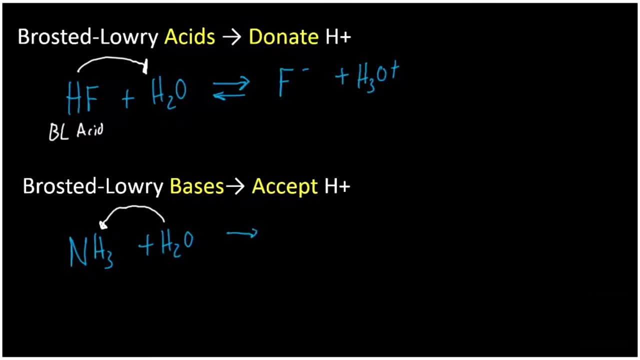 And so when ammonia gains a hydrogen ion, it's going to be transferred over to ammonia. When it gains a hydrogen ion, it's going to become positively charged and it's going to go from H3 to H4. So we get NH4+. Now what's left behind? Well, H2O right gave up a hydrogen. 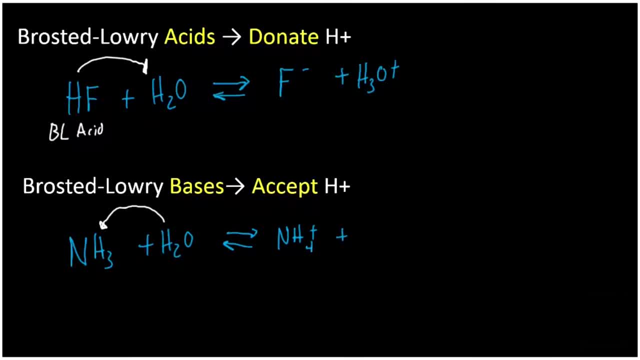 So it's going to become negatively charged and it's going to have just one hydrogen instead of two, So that's hydroxide. Now you might understand why NH3 is considered a base, because when you put it in solution, even though it itself doesn't have hydroxide ions, you can 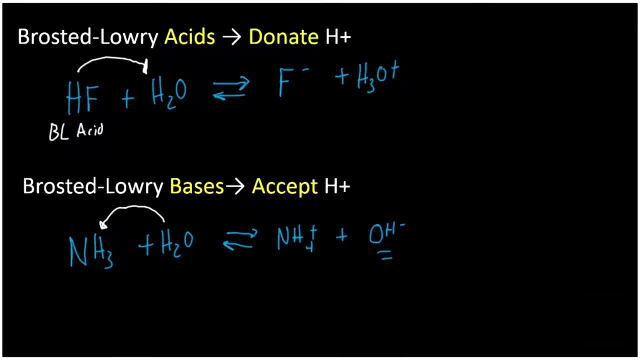 see that it actually does put them off into solution. So that means that NH3 is our Bronsted-Lowry base. Something interesting to notice here, though: In the top reaction water accepted a hydrogen ion. So in the top reaction actually there's a Bronsted-Lowry acid, NHF, and a Bronsted-Lowry 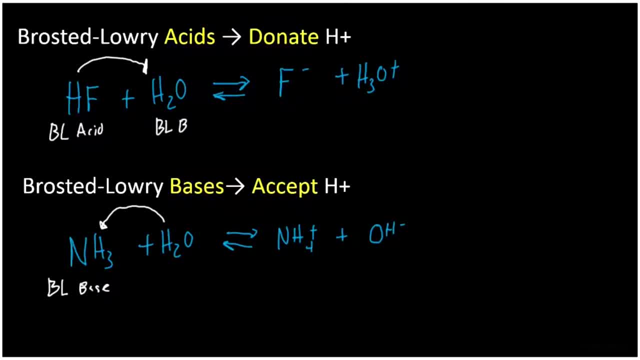 base in terms of water. So here we have a Bronsted-Lowry base. Why? Because one of them accepted a hydrogen, that's water, and one of them donated it. So the fact that our water accepted a hydrogen makes it a base there. In the bottom reaction, however, our water 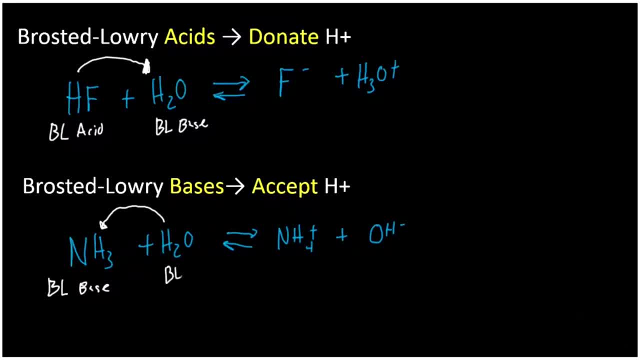 donated a hydrogen. That means down here it's acting like a Bronsted-Lowry acid. So that's a little different than what we've seen before with, say, the Arrhenius definition of an acid or a base. We're used to thinking of a given compound as either an acid or a base. 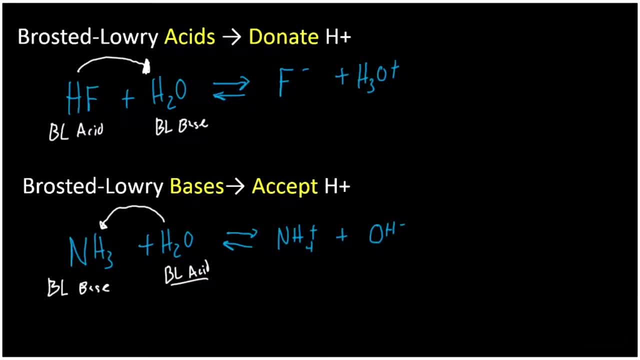 But we can see here that, based on what you mix water with, sometimes it's going to accept a proton, Sometimes it's going to accept a proton, Sometimes it's going to accept a proton, Sometimes it's going to donate a proton, And that makes it what's called amphoteric. 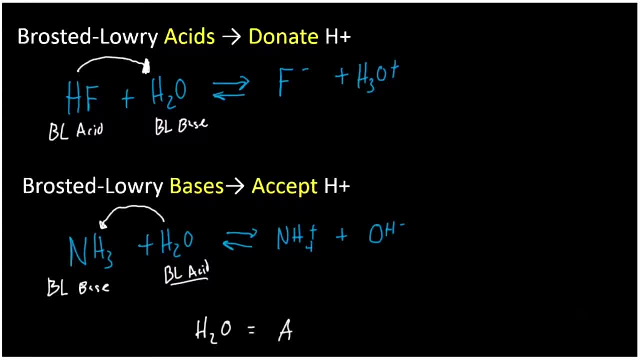 So H2O is amphoteric, And that means it can act as an acid or a base, Acts as acid or base. Okay, some other vocabulary that you should be familiar with when it comes to Bronsted-Lowry acids and bases are conjugate acids and bases. Here's the trick If you have a Bronsted-Lowry. 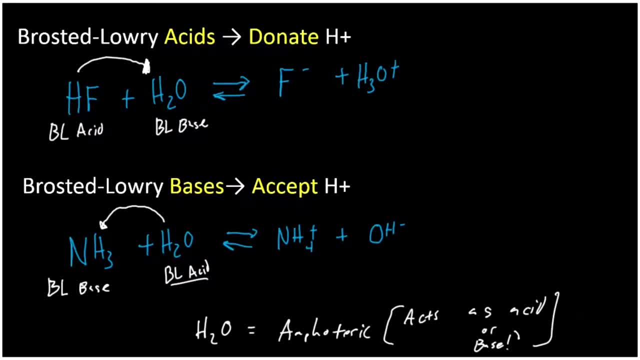 acid. After it donates a hydrogen, it becomes a conjugate base. So that means fluorine is a conjugate base. Why is it a conjugate base? Well, think about what fluorine would do. It's negatively charged. So if fluorine had to do something with a proton, it would accept. 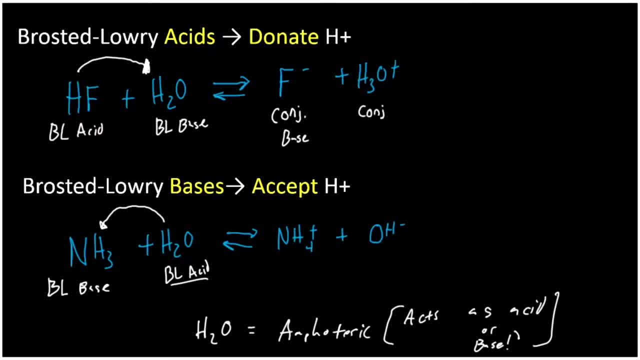 a proton. Meanwhile, H3O plus becomes a conjugate acid Because it now has an extra hydrogen, it could give up. So whatever was my Bronsted-Lowry acid becomes a conjugate base. Whatever was my Bronsted-Lowry base becomes a conjugate base. Whatever was my Bronsted-Lowry acid becomes. 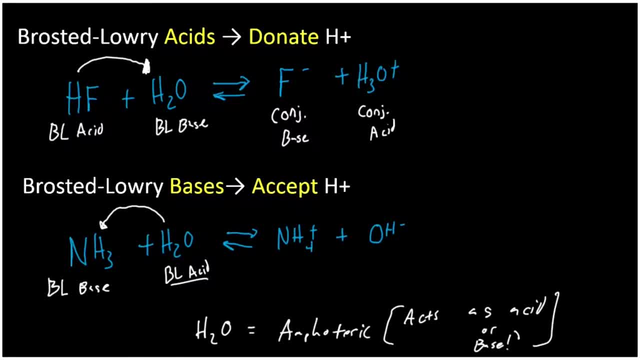 a conjugate acid. So it's important for you to be able to look at a reaction and identify the Bronsted-Lowry acid, the Bronsted-Lowry base, the conjugate base and the conjugate acid. Let's look at our bottom reaction. We had the Bronsted-Lowry base in NH3. that 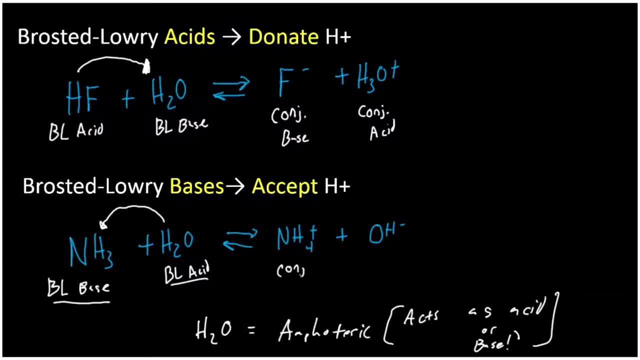 became NH4.. That's now our conjugate. What do you think? Acid or base? Well, it was a base, so now it's an acid. OH minus, on the other hand, came from water and now it's a conjugate base. That should make sense. If you ever labeled OH, you would think, oh, ok, this was an acid and now it's an acid. But when you look at the H3, it's a conjugate base. It's a conjugate. 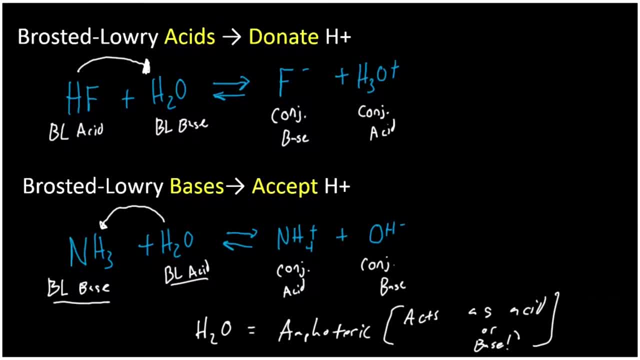 you ever labeled OH- an acid of any kind, you would know something was going wrong. Similarly, if you ever named H3O+ as a base of any kind, you would know that was going wrong. So we've introduced you to a fair bit of vocabulary on this page: Bronsted-Lowry acids and bases. 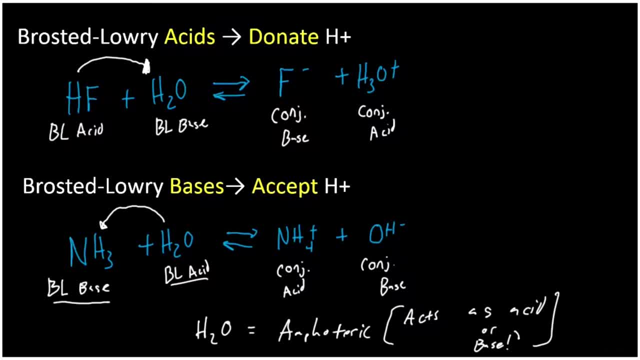 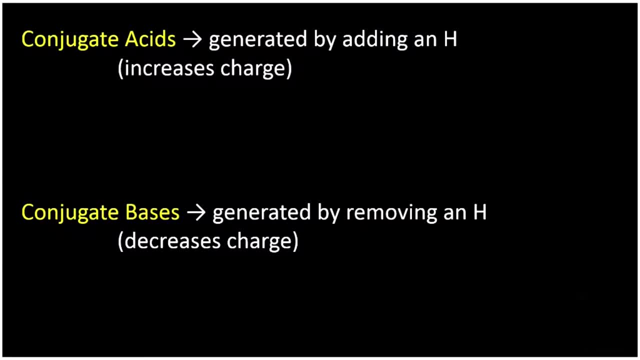 conjugate acids and bases and the idea that some compounds are amphoteric. Let's keep working with these ideas, All right. so one thing to keep in mind is: how do you generate a conjugate acid? Well, we make it by adding an H+. So, just like we saw in the previous slide, we generated 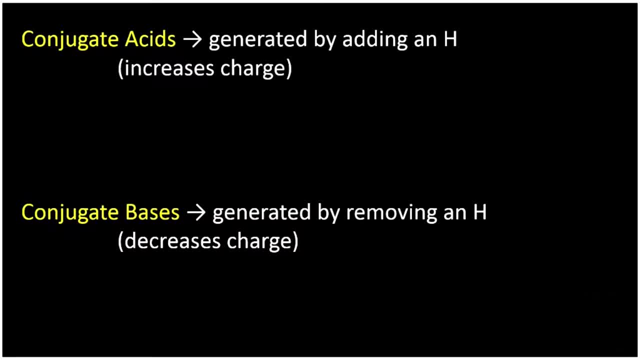 conjugate acids from bases that have gained a hydrogen. And so that means, say, we had H2PO4- And we want to know what is the conjugate acid of that guy. Well, the conjugate acid is generated by adding an H. So we got to add an H, which would give me H3PO4.. Now what's the charge? 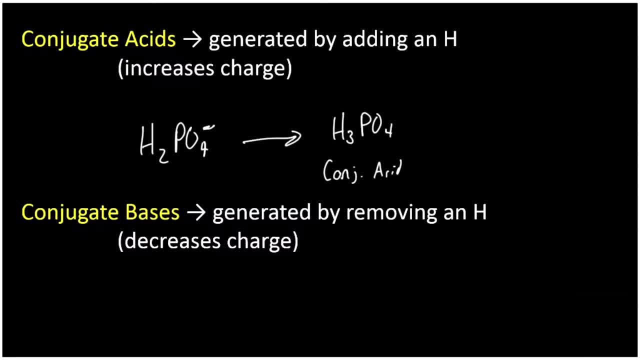 Well, before it was negative 1, and then I added plus 1 to it, And negative 1 plus 1 gives me 0. So that actually is a neutral charge. there, Conjugate bases are generated by removing an H, So we see: 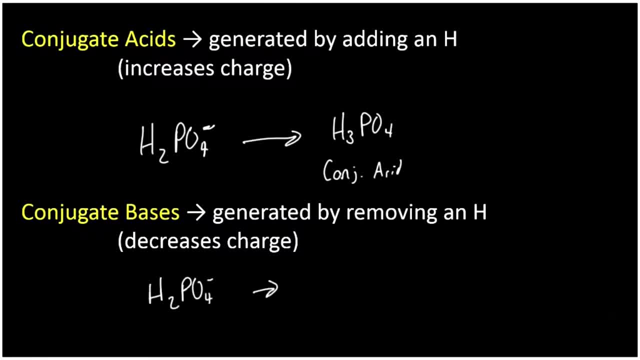 that H2PO4- can go to its conjugate base by dropping a hydrogen HPO4.. Since it lost something positive, it goes from negative 1 to now negative 2. And that's the conjugate base. All right. 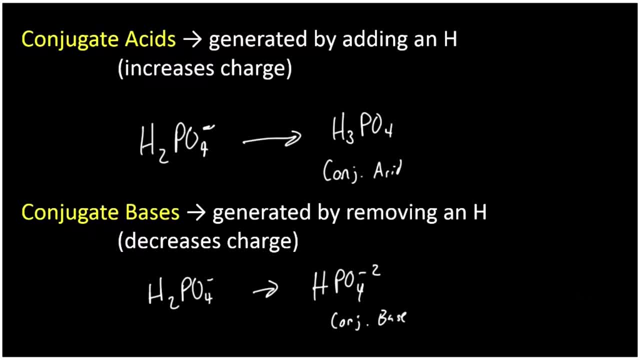 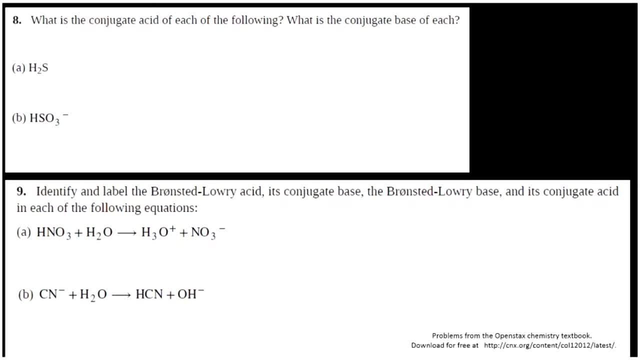 let's do a few practice problems with conjugate bases and acids and our Bronsted-Lowry and acid definitions. Okay, so these are both from the open stack textbook, And problem eight says what is the conjugate acid of each of the following? What's? 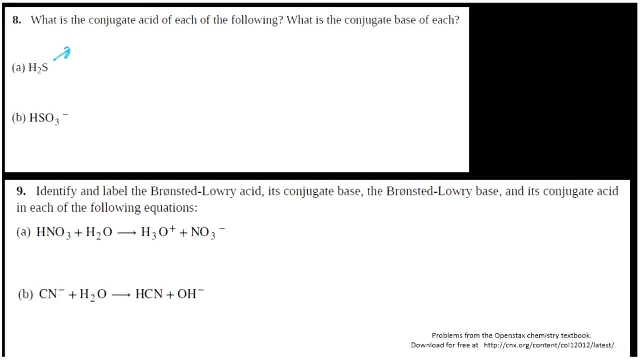 the conjugate base. Well, to generate the conjugate acid, remember that we add a hydrogen, So that would be H3S+. It becomes positive because it gained a proton, So that's the conjugate acid. On the other hand, losing hydrogen would make HS- the conjugate base. 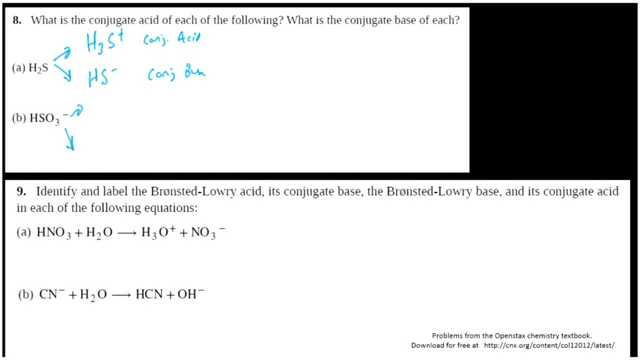 And HSO4,. similarly, if I wanted to make a conjugate acid, I add a hydrogen and it becomes H2SO3.. It neutral because it was negative 1, and it gained a proton. All right If it loses a. 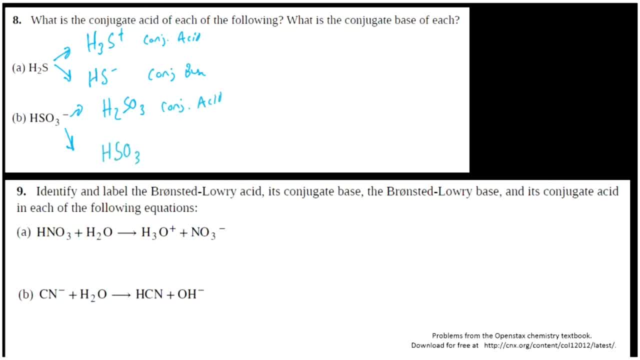 proton to become its conjugate base. it's HS03.. And now it's two minus because it's lost something that was positive. Okay, Last little problem here before we wrap up this lesson. Identify and label the Bronsted-Lowry. 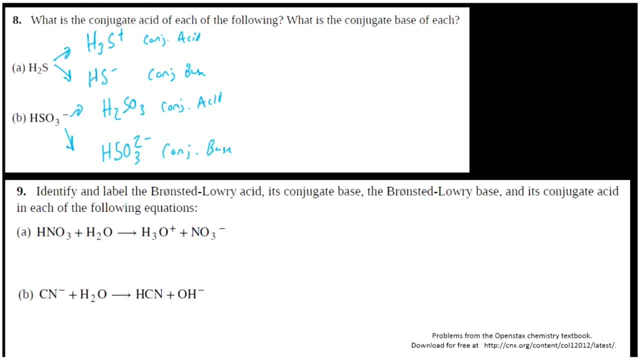 acid, its conjugate base. So okay, so we have the폰oid, Spanish's reinv, starred in a. now we're going to go over to Non's Bronsted-Lowry base and its conjugate acid in the following equations: All right, So what we want? 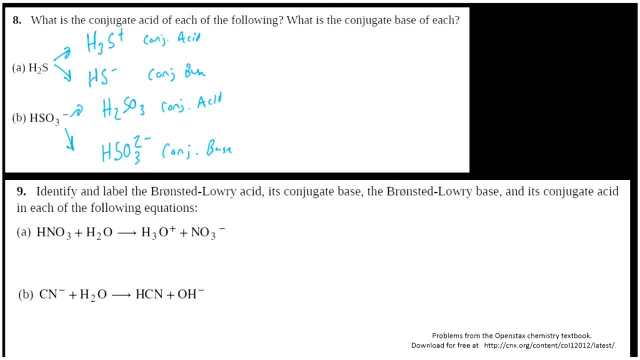 to think about is what of these is gaining hydrogen and what's donating? Here we see that we have HNO3, and then on this side, NO3- So what's that NO3 done? It's lost a hydrogen ion. It's donated it. So, since the hydrogen ion was donated from HNO3 to water, we know this is our